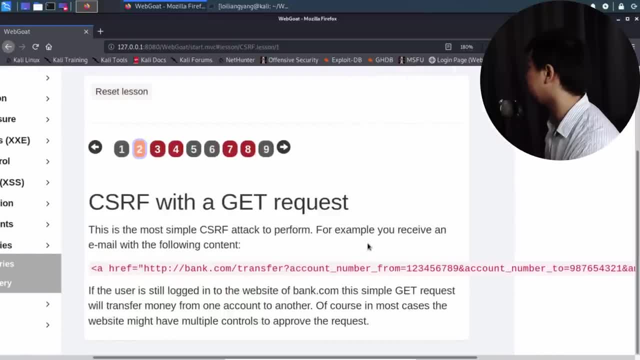 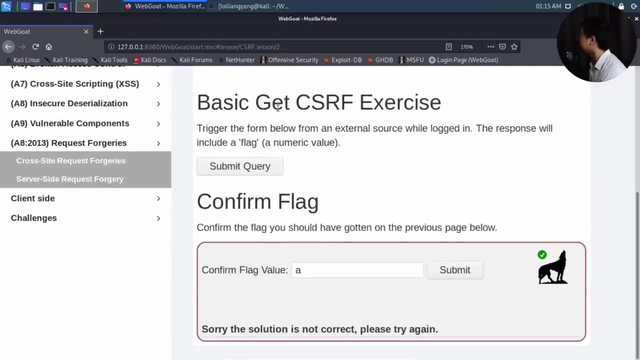 account number. So that's the whole idea behind it, and that's the whole idea behind how cross-site request forgery can be done with a simple get request. All we got to do now is look at the following. All right, so we have the basic get cross-site request forgery exercise. 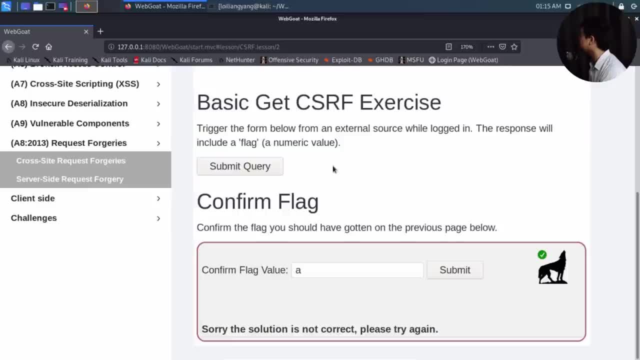 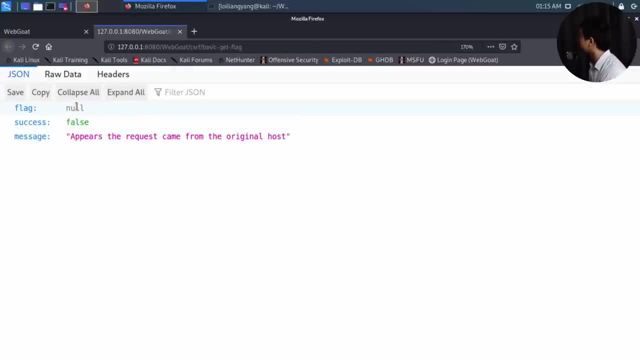 And if you trigger the form here from an external source, okay, and now we're on an internal source here, which is submit query. So if I go ahead and clicked on it, you'll see the following: Success false and there's a null for the flag and it states: on the left side appears the request. 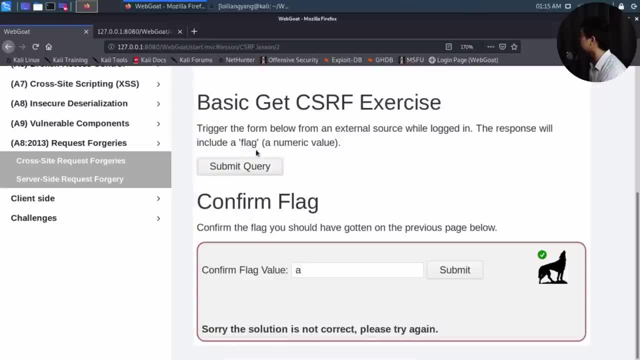 came from the original host, So the web form over here, as you can see, is hosted on the same IP address. that's hosting the web. good platform, All right. so what we can do next is to craft our own payload. So all we got to do is do a right click and do an inspect element. 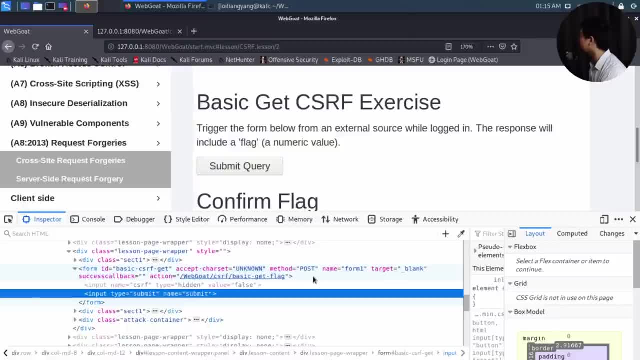 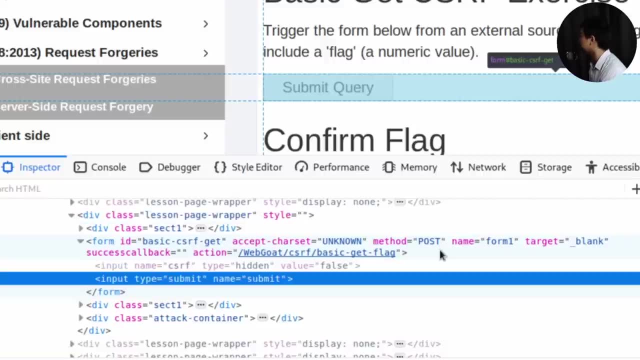 And see where exactly is the form going into. So on the bottom we have the inspector. All right, so in web developer you can use it either with your Firefox, with Chrome, whichever the browser it is, doesn't matter. Okay, you'll be able to see where we're taking action into And then 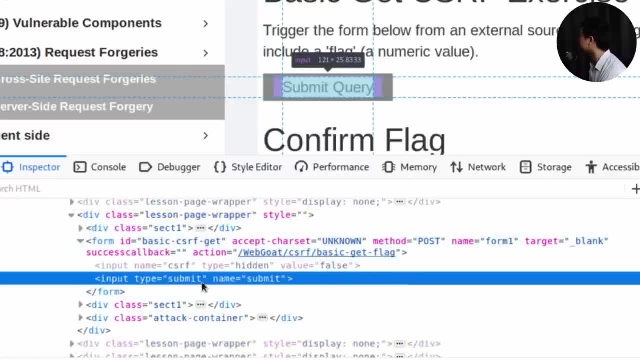 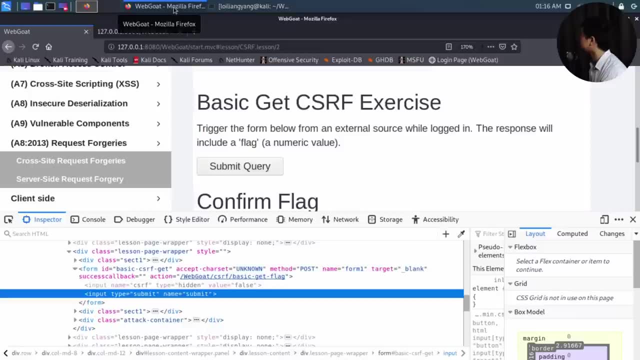 of course, there is a submit type, All right. so you have an input type here- submit, and the name is equal to submit And you end the form right here. as simple as that. So you can actually craft out your own form. So, in my case, what I'm going to do now is to show you the form that we 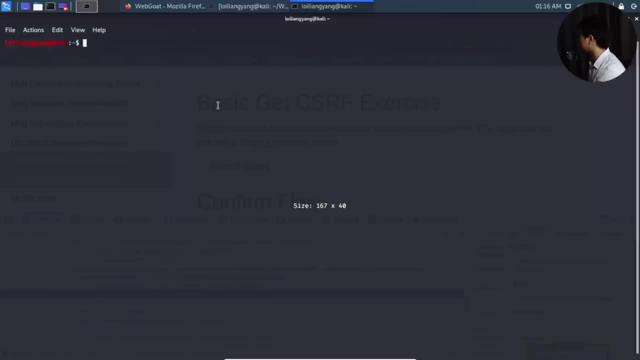 have crafted. So I'm going to go ahead and enter a terminal And we're zooming a little more so it's free to see, And I can go into desktop And I've already created a form to show and demonstrate to you how it looks like. So I can enter cat. all right, webgoat csrfhtml. hit enter on this. 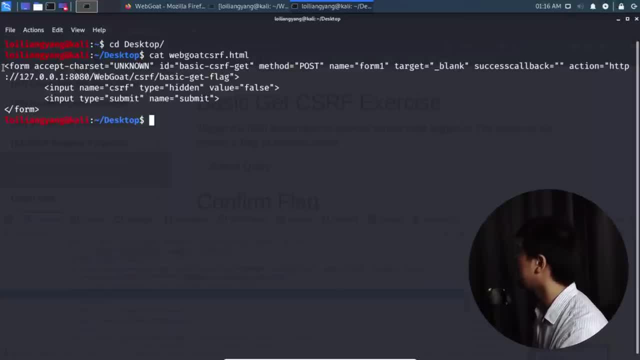 and we can see the form that we have crafted here. So we are following pretty much exactly what is needed in order for us to submit into the webgoat application server. So here we have the IP address of 127.0.0.1.. So of course, in the real world, on the internet domain you would have to specify. 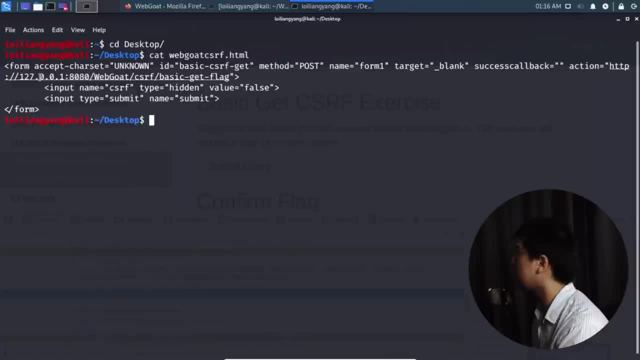 the domain name of the website, All right, so it could be e-commerce, science, social media platform, whichever the case is, And, of course, here we have the same input type- submit, equals submit- and the same input name here: csrf. 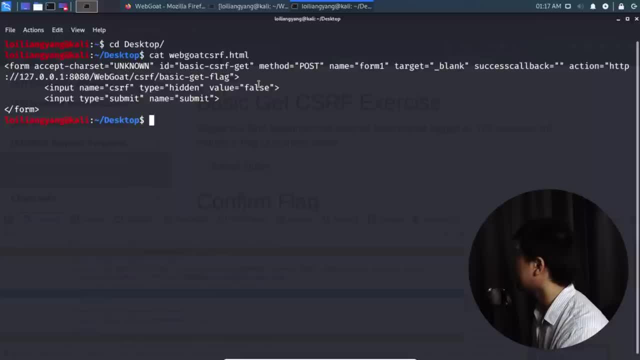 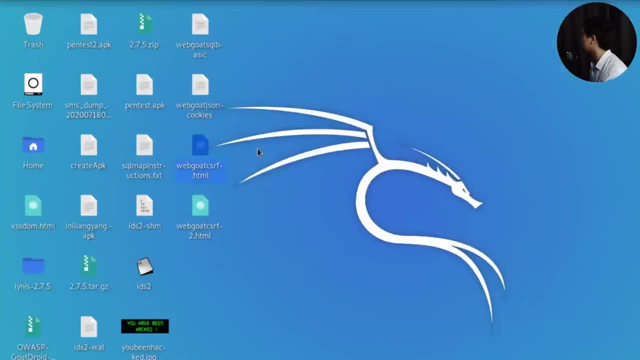 And of course, this is a hidden and value equals false. So once you have set all this forward, all right, you can actually go ahead and open up the file. So here I'm on the desktop And, of course, you can see a lot of payloads that we have created in regards to web application penetration. 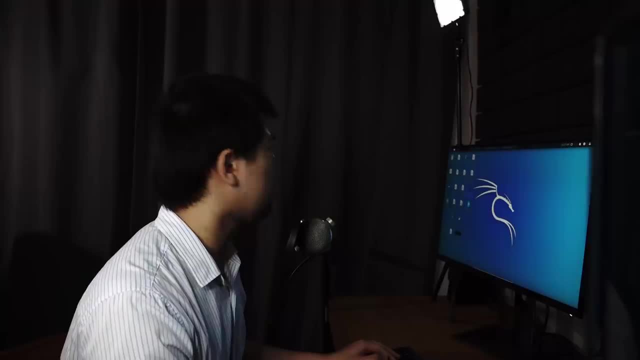 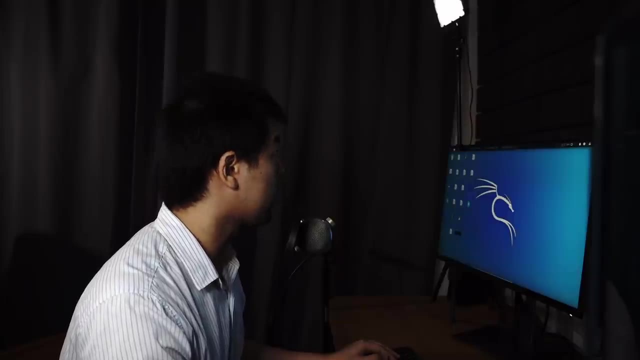 testing in regards to penetration testing and ethical hacking as a whole. So I really encourage you to subscribe to the channel so that you can be kept abreast of all the latest cybersecurity tutorials that we have And, of course, turn on notifications so that you can be. 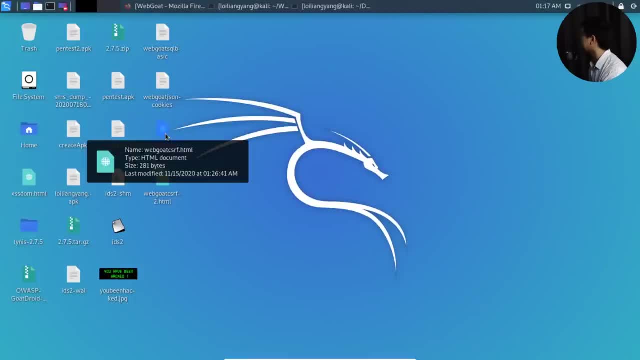 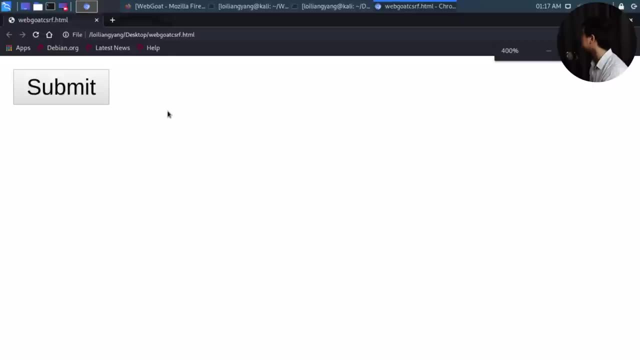 informed immediately when new tutorials come up. All right, so I'll go ahead and double click onto the following. So here we have webgoat csrf, right, double clicked on this And we can see right here: okay, we got the following file. So all I got to do now is go ahead and click submit And, of course, 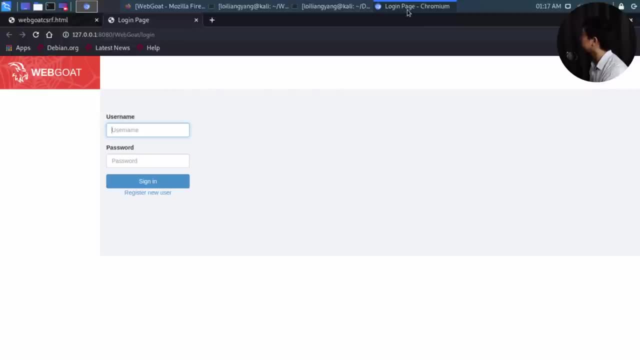 you see a problem here. that's happening And we're on a completely different browser, which is why it's not working. However, if I was to go back here and I copy the file, okay, copy the file. go back to the Firefox browser in which we are logged in as the user. I open a new tab. 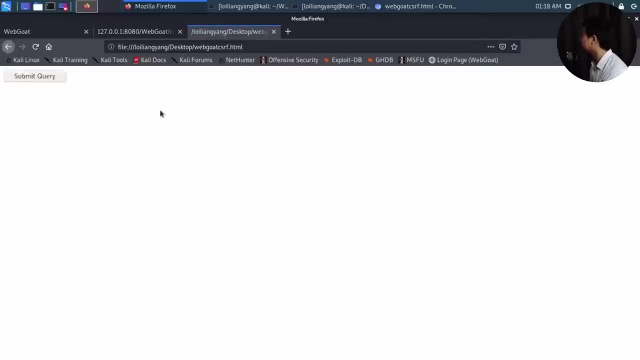 I paste it right here and I hit enter, And now we're back onto the same file And I click submit query. That's it, congratulations. appears you made the request from a separate host. So that's as quickly as that. we're able to launch the attack by using a separate form. The next question is: 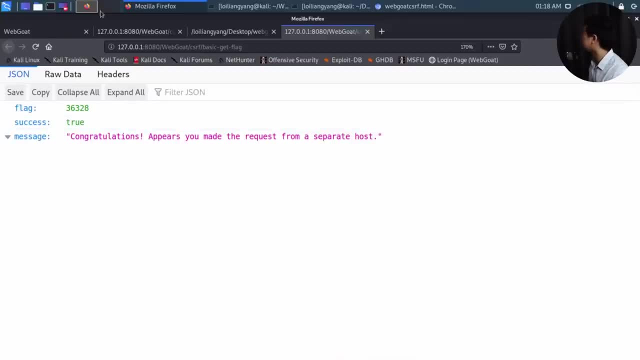 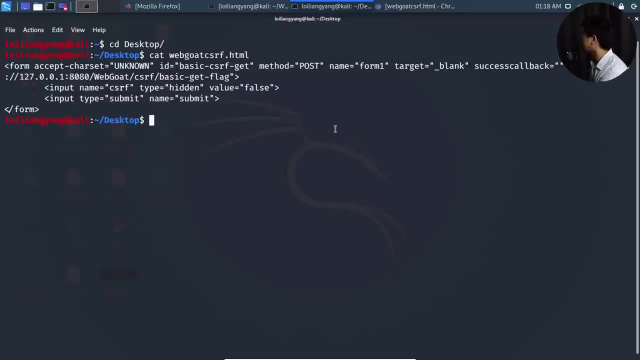 how can we take this to the next level? All right, so if I go back into the platform here, what I can do now is to go ahead and copy the file. All right, we can copy the file over webgoat csrfhtml that we just created and I can paste it to our own web application server. 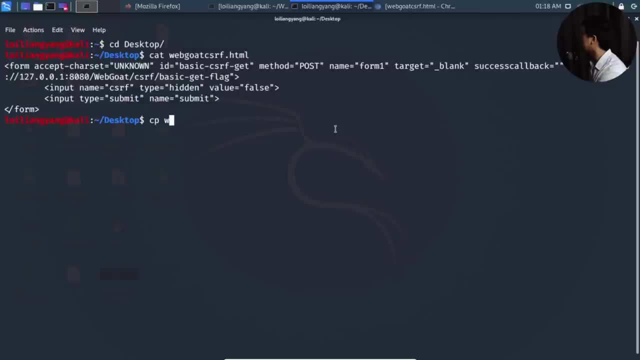 and we can host it very quickly. So what I can do is just go ahead and copy webgoat. all right, csrfhtml, and I copy the var wwwhtml and I hit enter on this And of course, we get permission denied. So no worries, enter, super user. do hit enter on that. 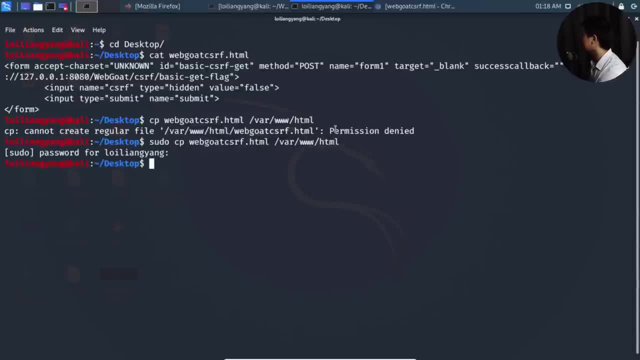 enter the password for a user account. Once we do that, we will now be able to say: list var- wwwhtml. hit enter on that too, And now we got a file right there- webgoathtml- csrfhtml- And I can navigate. now all right to the application server that we've created. 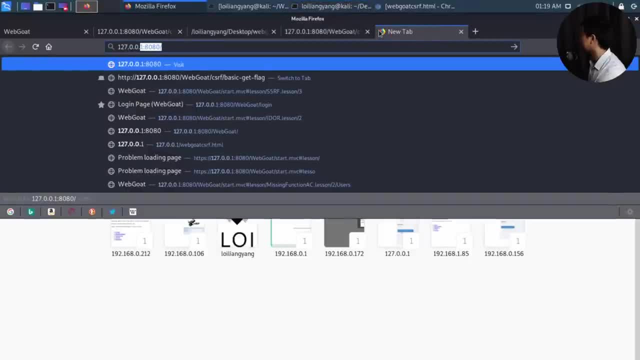 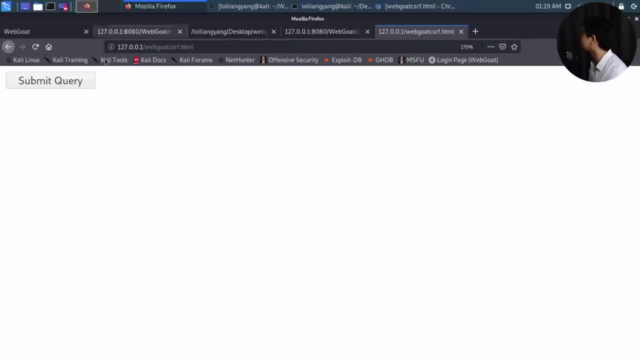 So I can go into 127.0.0.1, all right, followed by slash webgoat, csrfhtml, Hit enter on this again, And now we have hosted our hacking server, which has the fake form. All right. so all I got to do now is click submit query, And likewise we're able to get the flag.